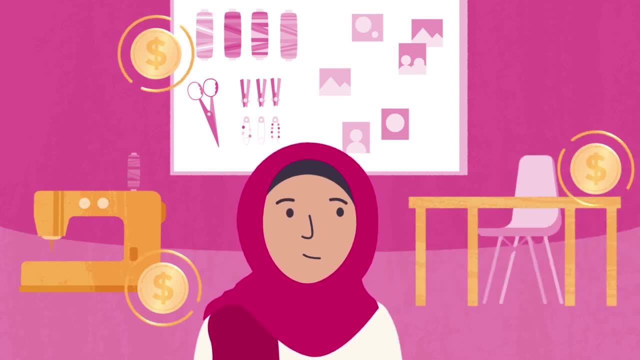 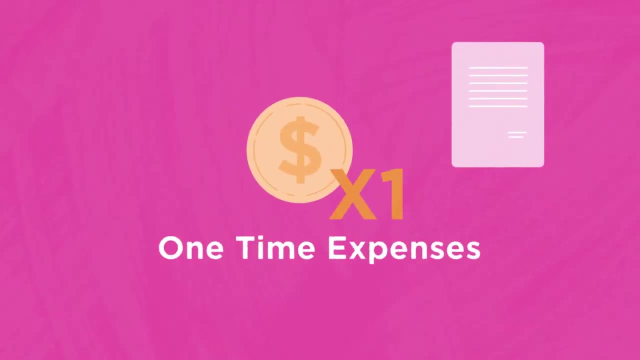 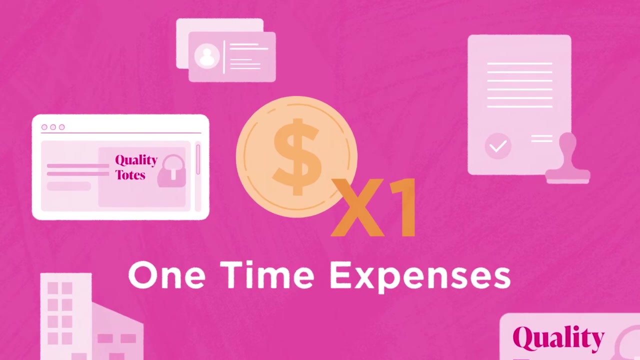 Knowing these costs allow you to know how much cash you should have in the bank before starting your business. Here are a few examples of startup costs: One-time expenses such as permits, licenses, registration fees, logo design, business cards, website down payment on rental property and leasehold improvements. 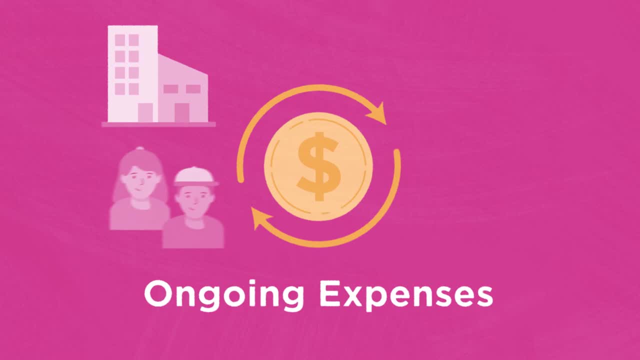 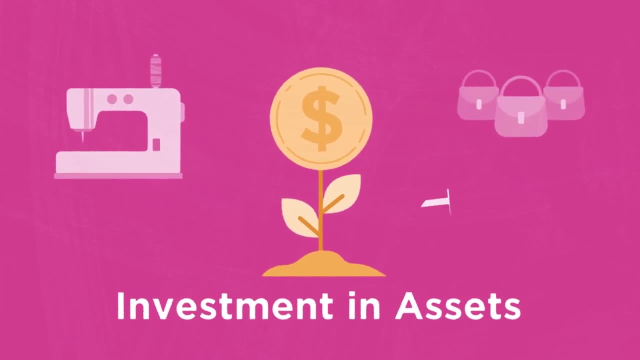 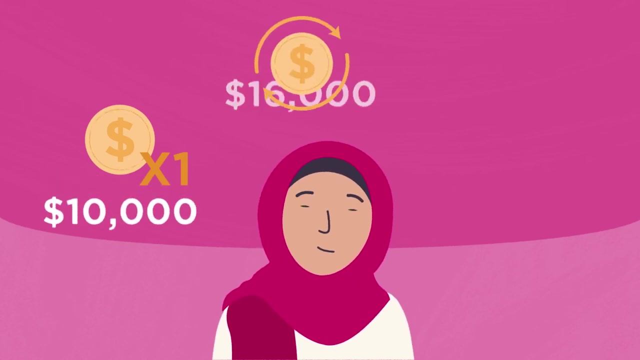 Ongoing expenses such as rent, payroll taxes, accounting services, insurance, utilities, Investment in assets such as equipment, inventory, furniture and vehicles. Finding these costs will allow you to know how much money you need to personally invest and or finance your business. 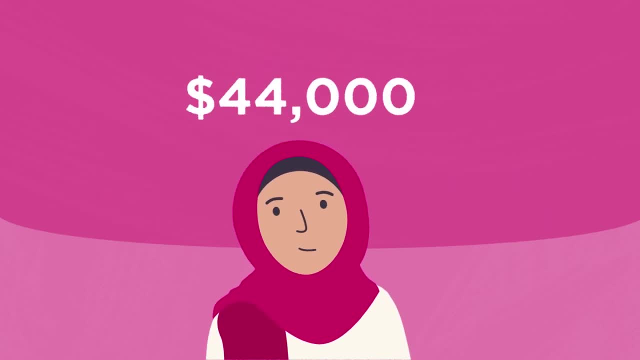 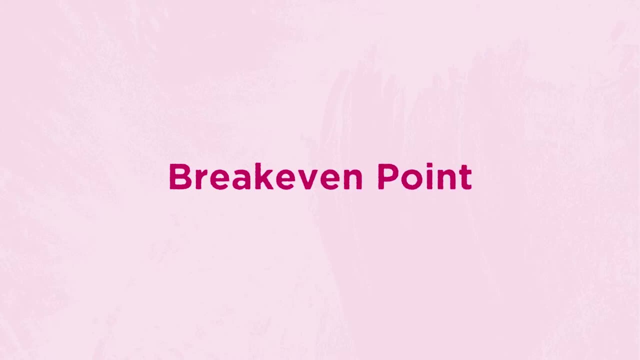 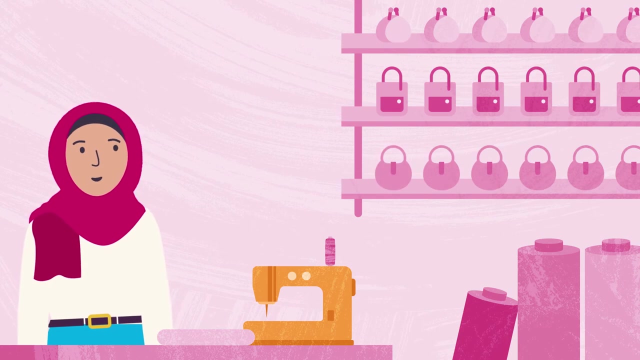 Just add them all up and you have your number. See, that was easy. Our final concept is the break-even point. So you want to start recovering your costs, paying your expenses and generating a profit from your business. You will need to know how many products and services you must sell and at what price you need to sell them at. 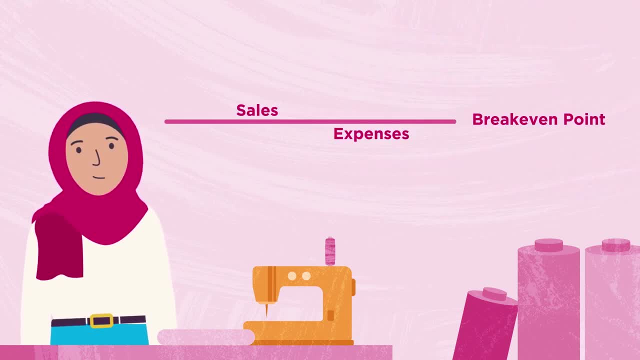 To do this, start by understanding your company's break-even point. The break-even point is the point at which your sales will exactly cover your expenses. Determining the break-even point allows you to know the level of sales needed to cover all costs and start earning a profit. 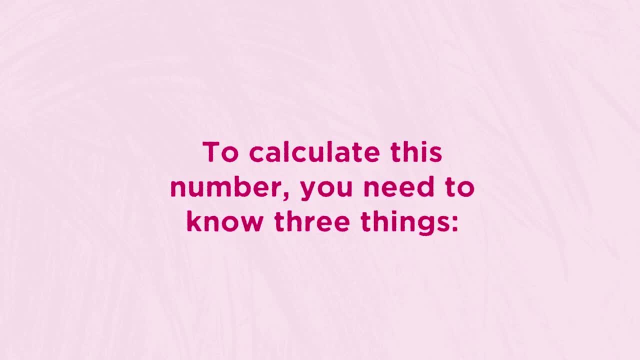 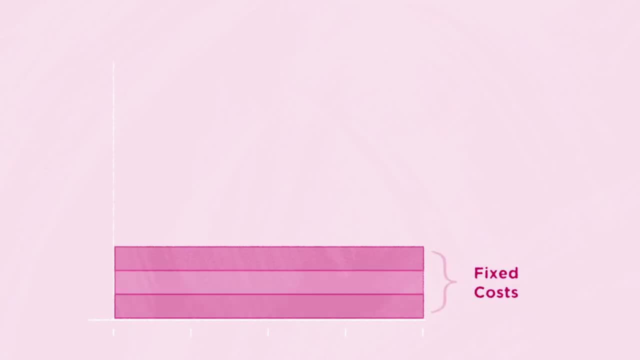 To calculate this number, you need to know three things. Fixed costs are costs that your business pays, whether you have sales or not. These items include rent, taxes, salaries and any other monthly expenses that do not change Whether you sell one product or 20, you still need to pay these expenses. 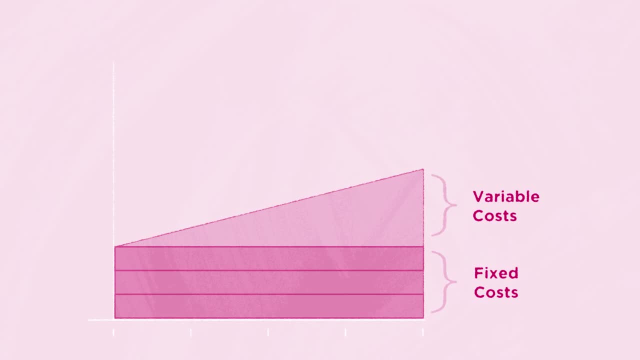 Variable costs are costs that change based on your number of sales, For example, raw materials, factory labor and sale commissions. Finally, you'll need to determine your selling price for your product or service. Remember whether you're just starting in business or creating a new product or service. 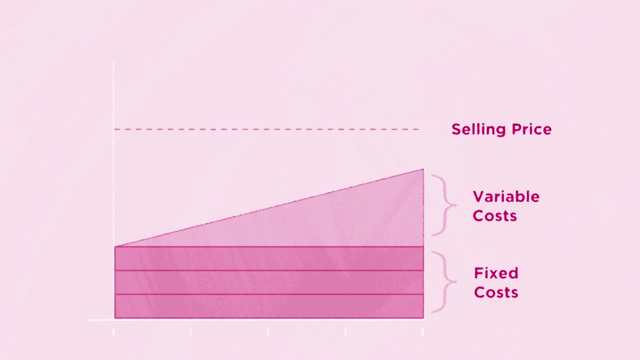 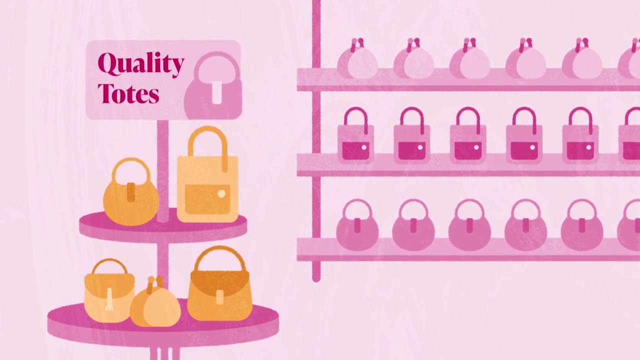 line for an existing business. you can adjust this selling price up or down as you start to calculate. Here's an example: Quality Totes Limited is a new company wishing to produce designer handbags. The company has calculated that it has fixed costs that can.